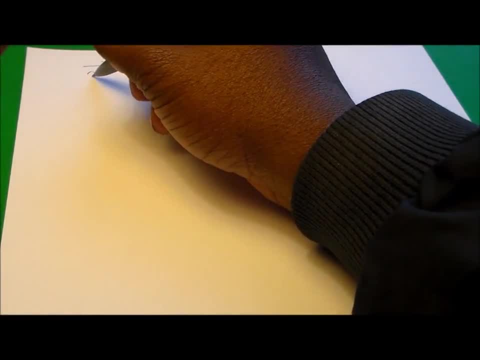 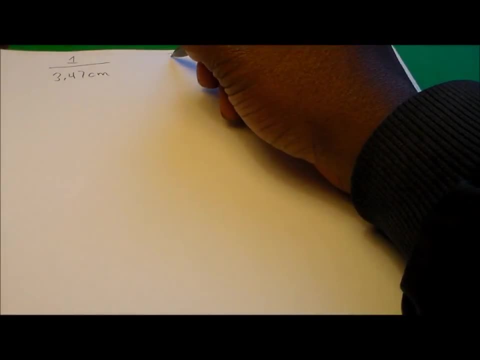 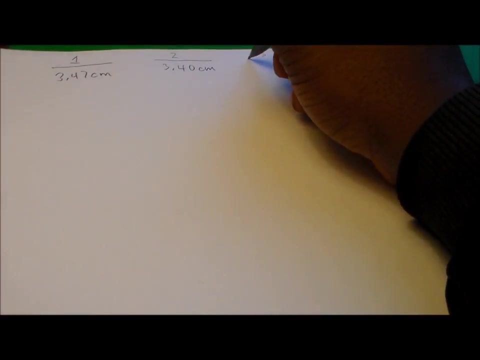 let's say, found that that item was equal to 3.47 centimeters. Okay, And then student number two measured the same item and figured that the item was 3.40 centimeters. And then student number three- the final of the three students, took the same measurement of the. 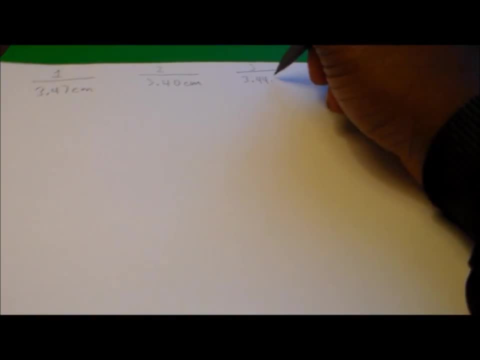 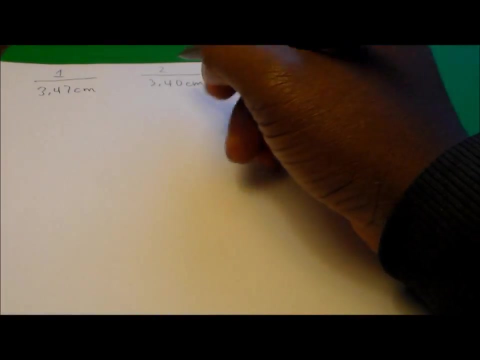 same item and that student thought that the item was 3.44 centimeters based off of the measurements. So one of the things that you'll notice here is that, with a high degree of certainty, the students can actually say they're very certain about this, or pretty certain. 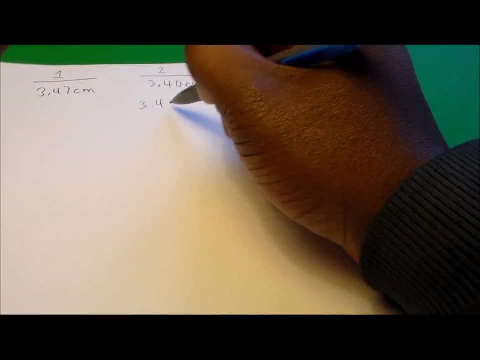 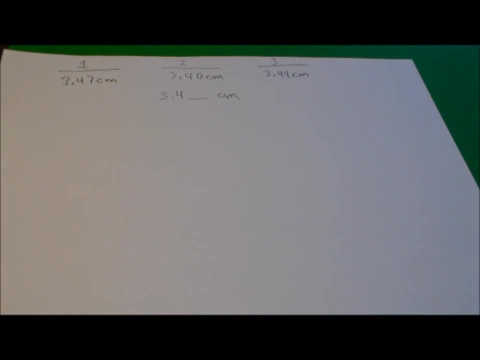 that the item that they're measuring is actually 3.4 something centimeters. Okay, 3.4 something centimeters. So how do we go about actually expressing the uncertainty related to this second digit after the decimal point? How do we go about actually expressing it in a? 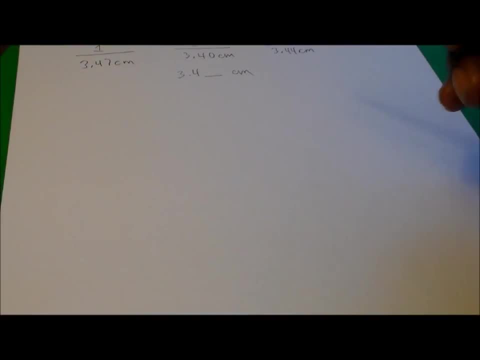 scientific way. Well, one way to go about doing so is to take the standard deviation of the three measurements here in order to figure out what the uncertainty is for the measurement that was taken. All right, The uncertainty equation is equal to: or, to be more specific, the standard deviation equation is equal to: 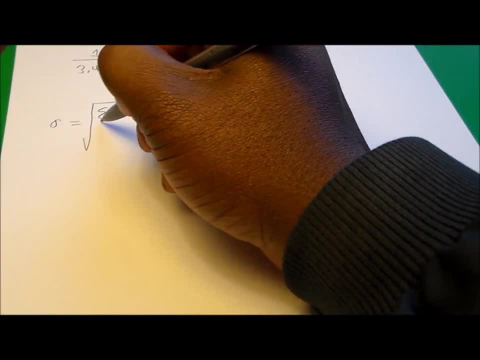 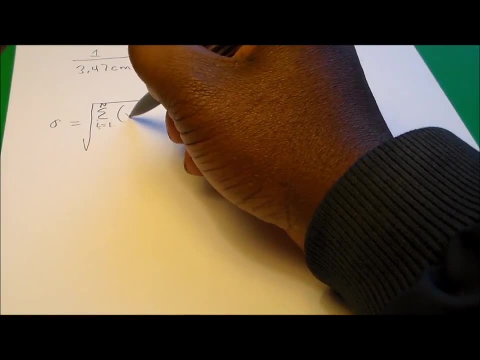 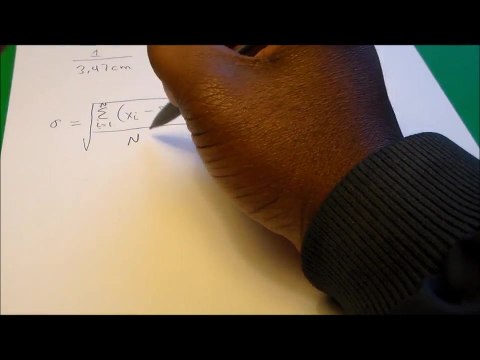 the square root of the following: the summation from sample one going to n, so that's i, is equal to one going to n Of x sub i minus x bar, which is x average squared all divided by the number of samples. 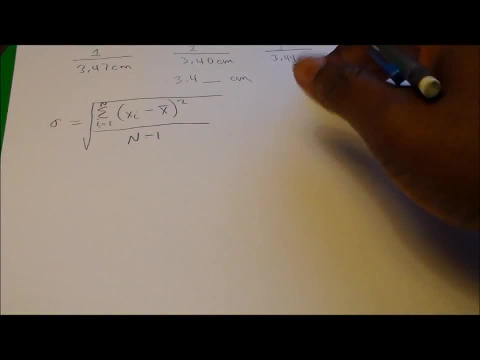 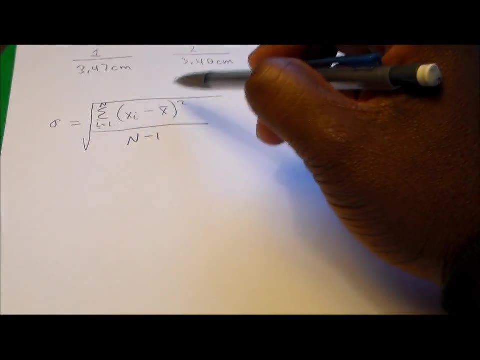 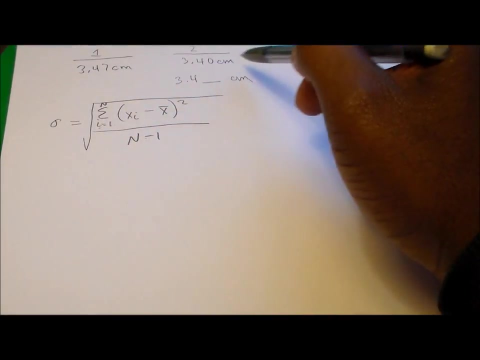 minus one, the difference between of that. Okay, So this sigma here, if you're not familiar with, means a summation of this number, this difference squared from of the total one through n number of samples. So in our case n is equal to three, because we have three. 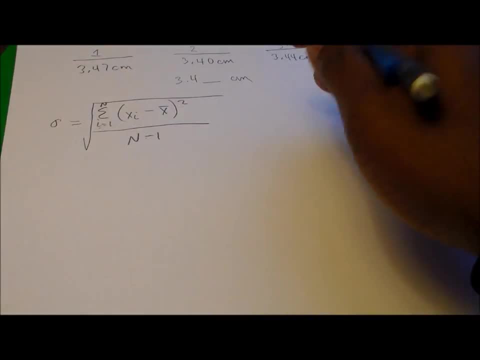 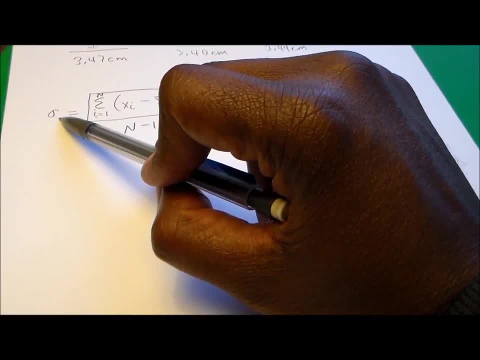 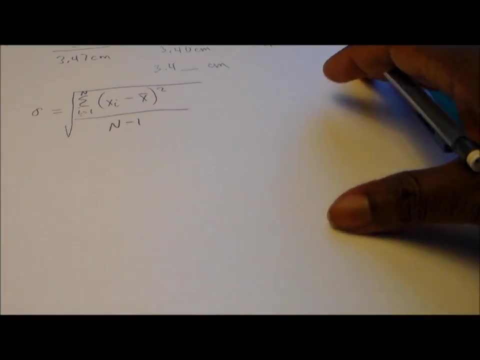 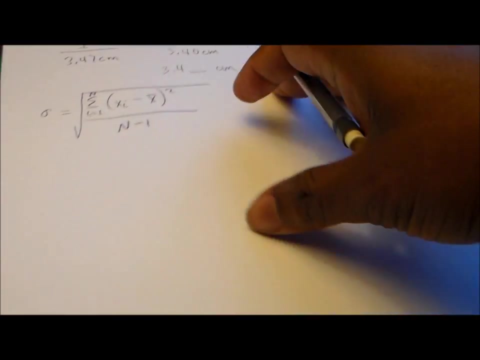 go about finding that uncertainty here, Which? that uncertainty is related to that last digit that we're not quite sure about. Okay, So, in order to find that uncertainty, what we're going to need to do is first find the x average, and, as you know, x average is equal to x one plus x two plus x three. 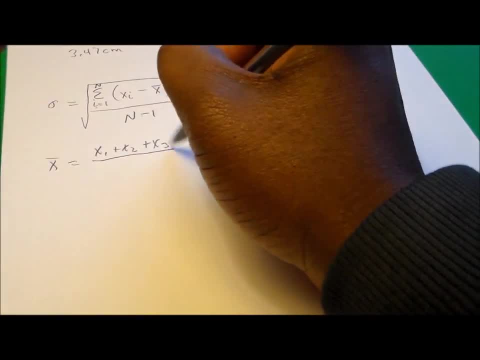 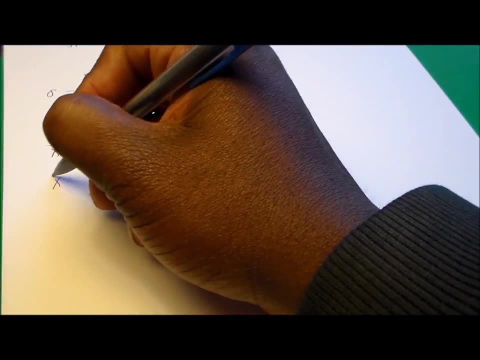 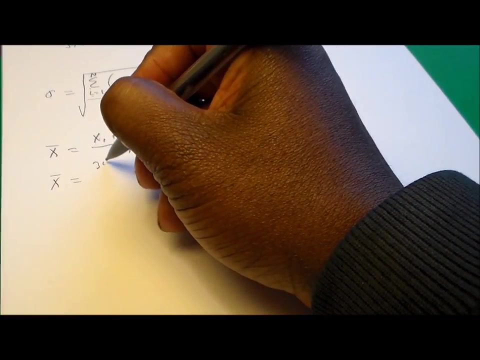 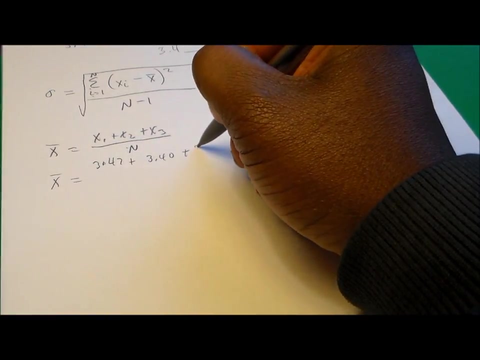 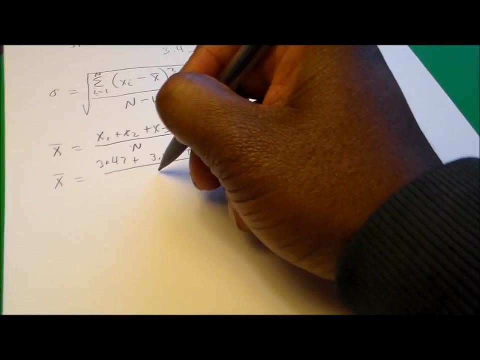 three, because we have three samples. so we stop there. divided by the number of samples, okay, and in this case the number of samples is three, and so that x bar then is equal to, and we add those numbers up, 3.47 plus 3.40 plus 3.44, divided by the number three here, and so we end up with then: 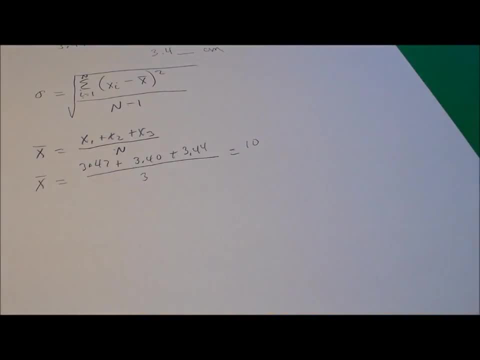 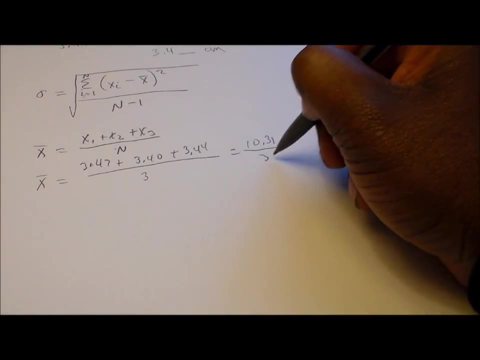 that this is equal to- and you can go ahead and calculate this out. I already did. it turns out this is equal to 10.31 divided by the number three, and when we actually calculate at 10.31 divided by number 3, we end up with 3.44 centimeters. if we 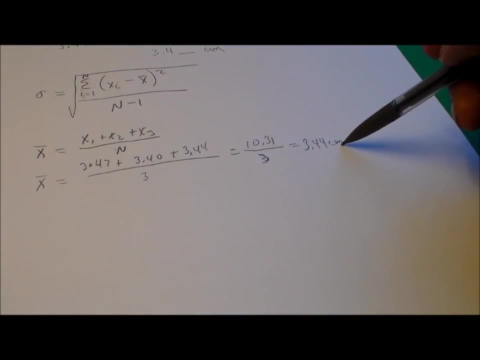 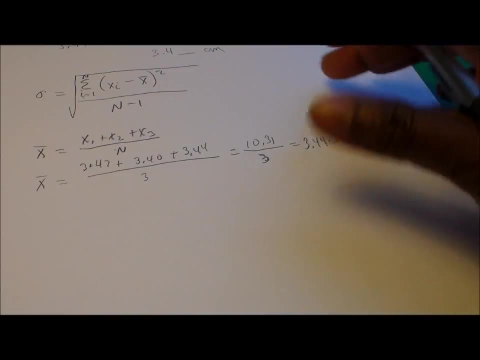 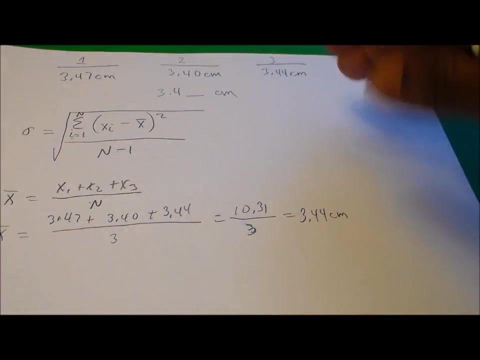 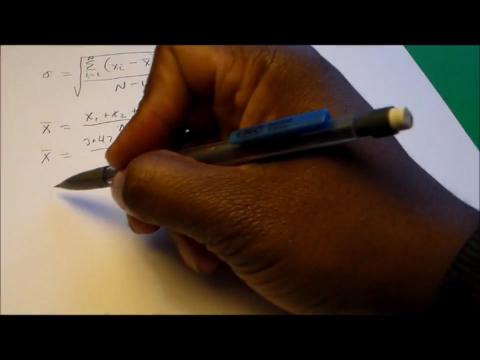 pay attention to our significant figures, we end up with 3.44 centimeters. alright, so that's our average, or x-bar. So now what we need to do is we need to take that average and subtract from each of those the samples that was collected. so start with sample number one. start with sample. 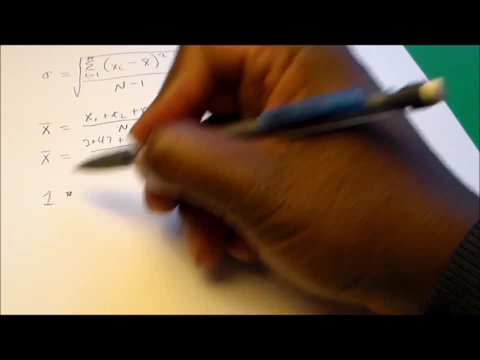 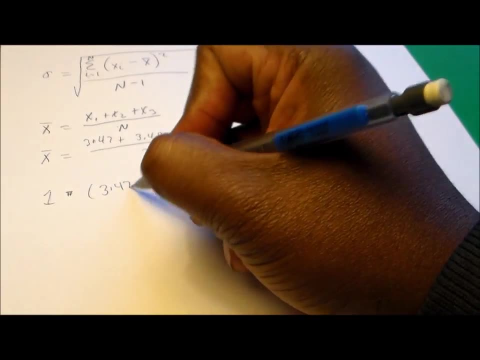 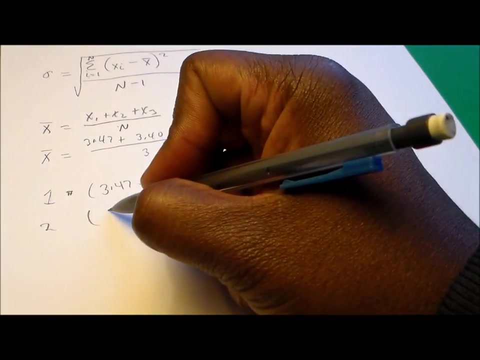 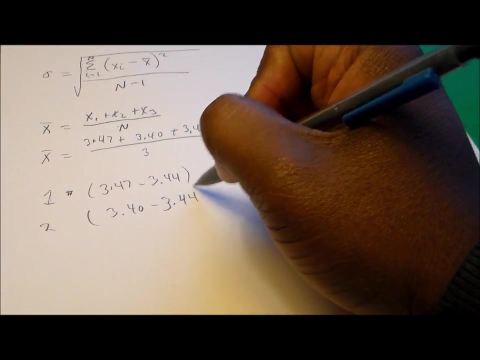 number one. student number one found that. let me not use an equal sign there. student one found what was it? three point four, seven minus the average, which is three point four, four. student number two: three point four, zero minus three point three point four, four. and student number three found three point four four. 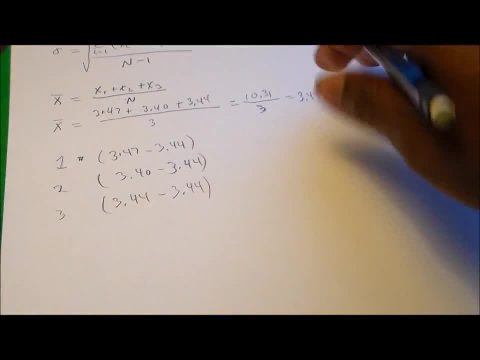 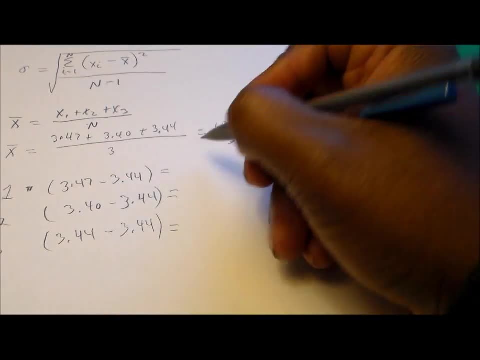 and we're going to subtract three point four, four from that. okay, so what we end up getting here then, when we take the difference, is we end up with zero point four, four. and we're going to subtract three point four, four from that. okay, so what we end up getting here then, when we take the difference, is we end up with zero. point four, four, and we're going to subtract three point four, four from that. okay, so what we end up getting here then, when we take the difference, is we end up with zero point four, four, and we're going to subtract three point four, four from that. okay, so what we end up getting here then, when we take the difference, is we end up with zero. 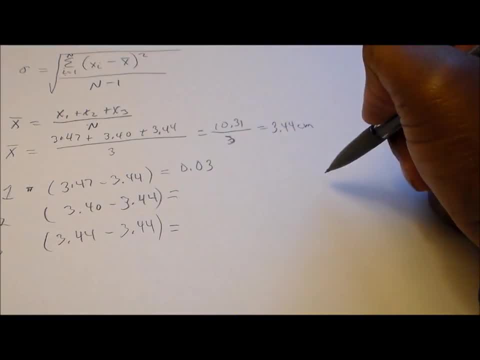 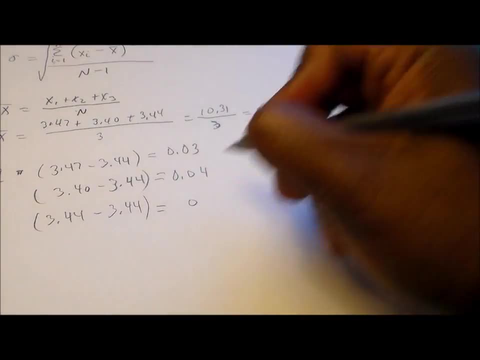 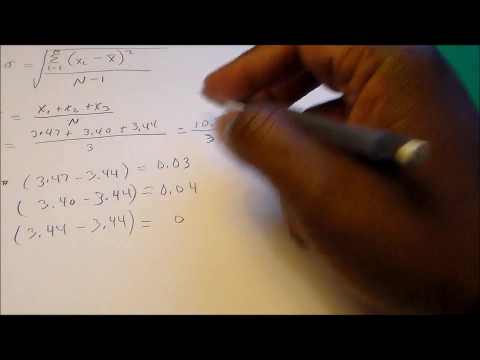 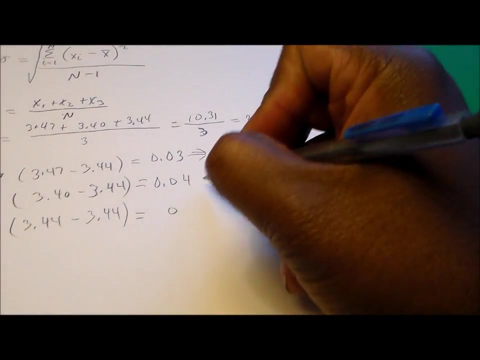 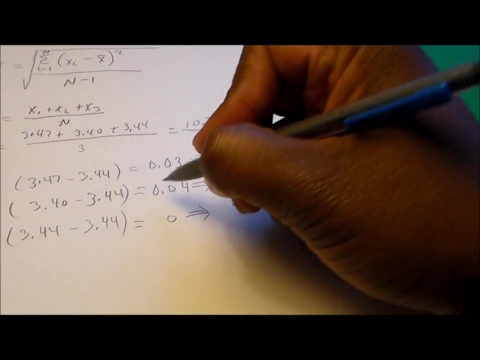 point zero three, okay, and we end up here with zero point zero four, and we end up with zero in this case. okay, If we now remember, we said we needed to square those differences, right? so we now have to square all three of these, so that's zero point zero three, and this should be negative. I forgot. 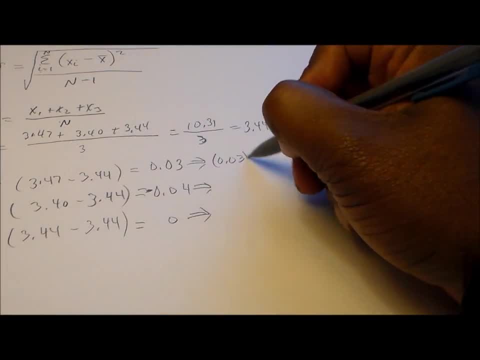 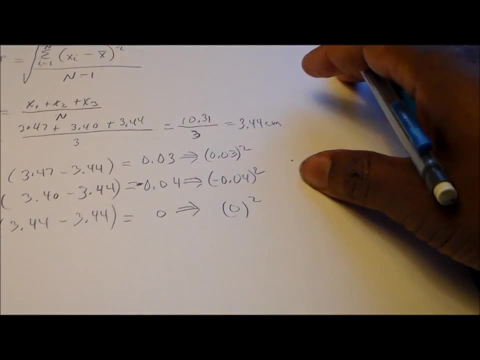 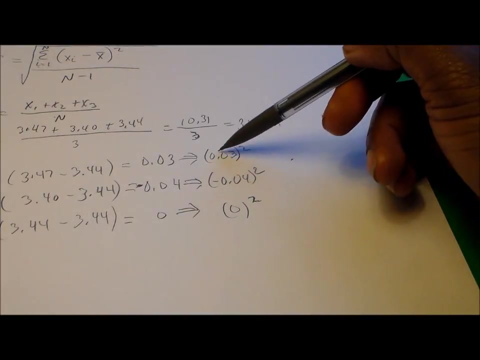 the negative sign there. sorry about that. This should be zero point zero three squared. this should be negative: zero point zero four squared, and of course this is zero squared. all right, We have one significant figure here. one significant figure here when we do zero point zero three. 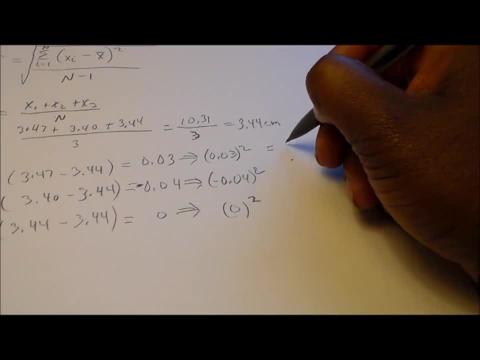 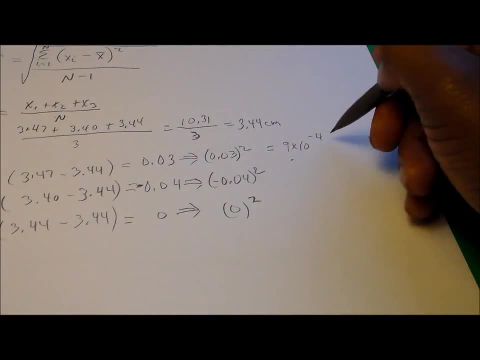 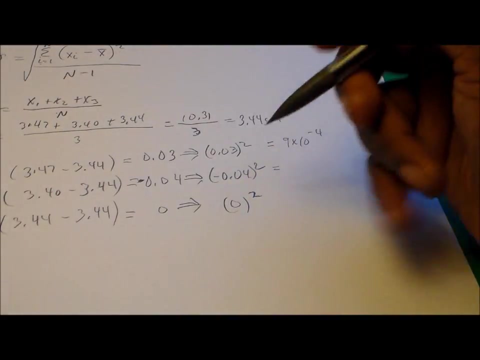 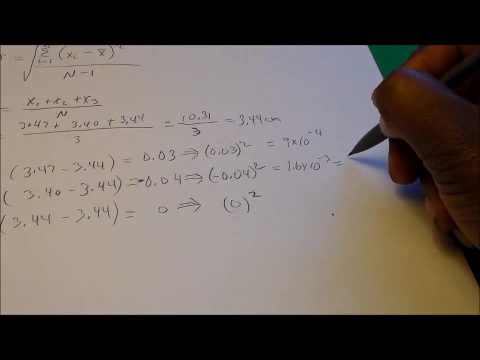 times zero point zero three, We end up with nine times ten to the minus fourth, with one significant figure, okay. and when we do the negative zero point zero four, we square that, we end up getting one point six times ten to the minus three. but because of significant figures we'll go ahead and 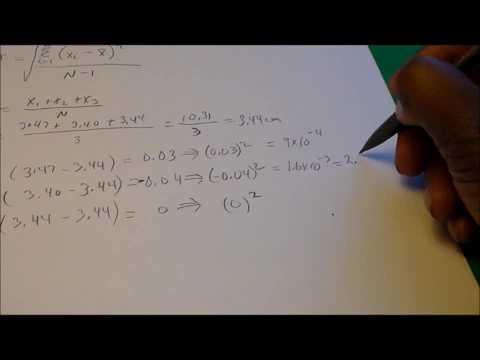 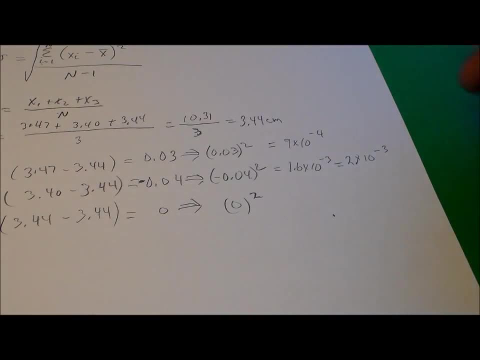 make that two point, or, pardon me, not two point, but two times, Okay, Ten raised to the minus three. okay, so that's two times ten raised to the minus three, and let's go ahead and move this across. so it's nine times ten to the minus four, and then 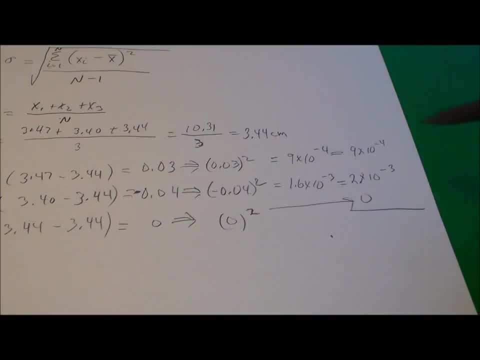 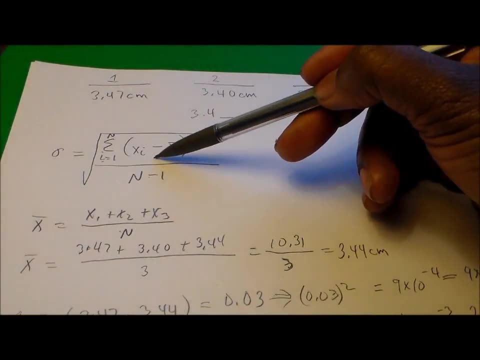 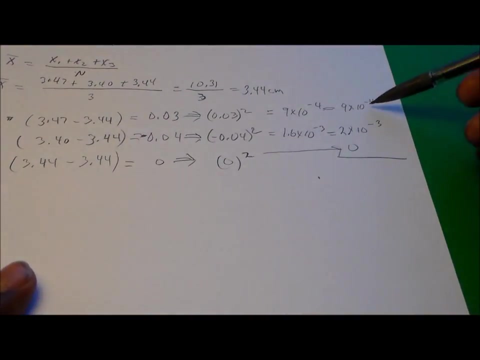 of course, this is zero. okay, so now we have our three squared differences. all right, Now, according to our calculation here, we now need to sum them all up, Okay, So when we sum all three of them up together- and this one I'm going to do on the calculator, 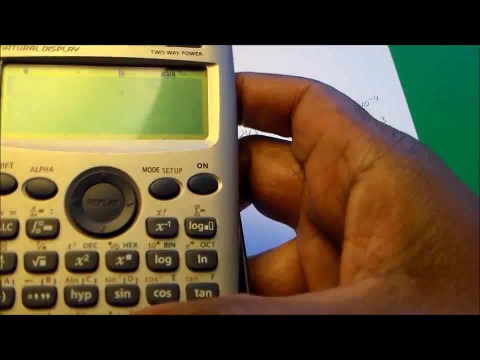 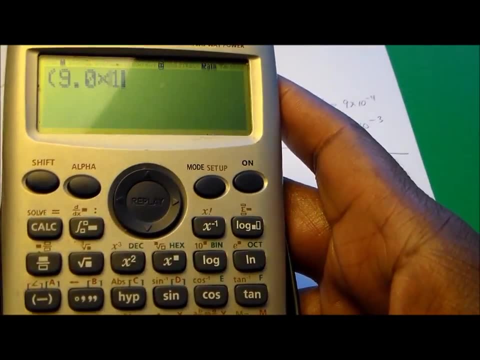 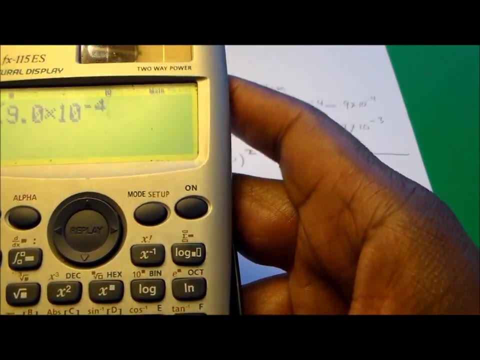 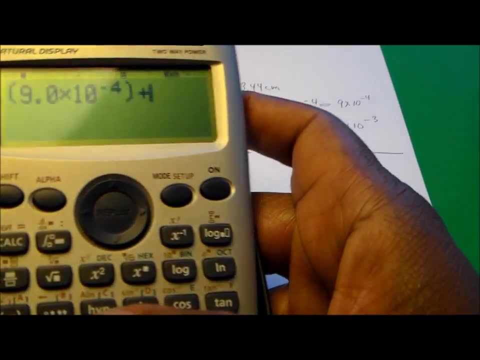 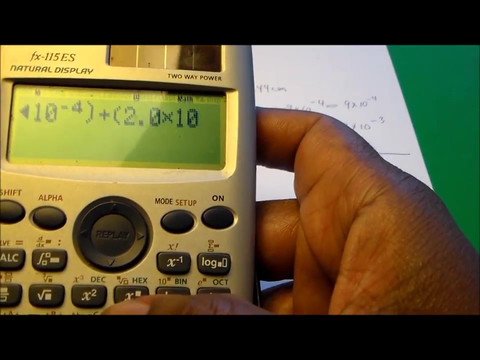 on the screen here so that you can see how this is done. we're going to start by opening parentheses, and that's going to be nine point zero times ten, raised to the minus four. okay, Close parentheses, Okay. Close parentheses, Okay. And then we need to add that, to open parentheses, two point zero times ten, raised to the minus. 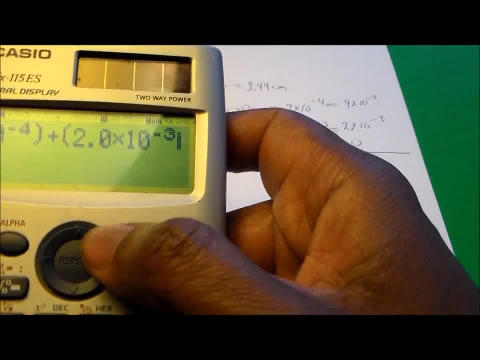 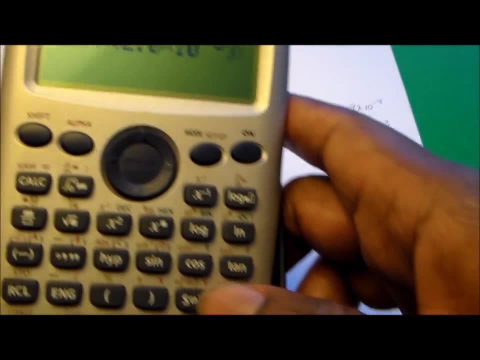 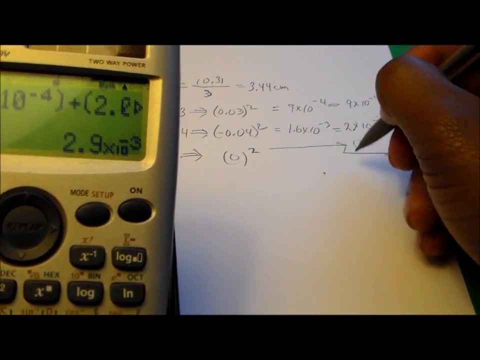 three, and then we move that across and close parentheses, all right. so we end up having this on our screen and some of it is actually over here that got cut off and we say we want to equal that, Okay. So we're going to start off with two point nine times ten to the minus third, okay, two. 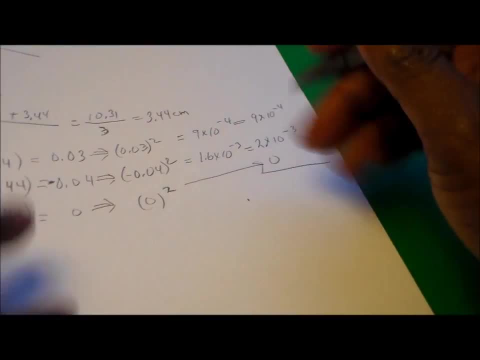 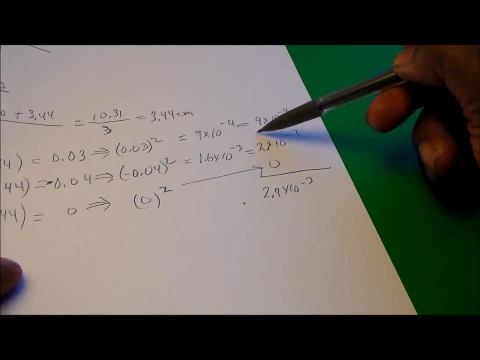 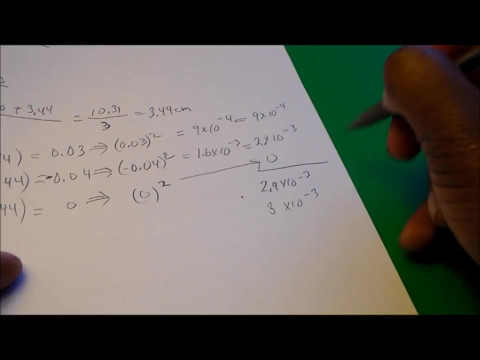 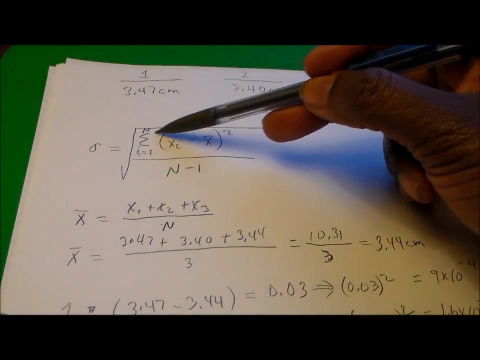 point. nine times ten to the minus third. okay, but paying attention again to our significant figures, we go ahead and change that to approximately three times ten to the minus third. okay, so three times ten to the minus third, okay. going back up here now, so we've done everything in. 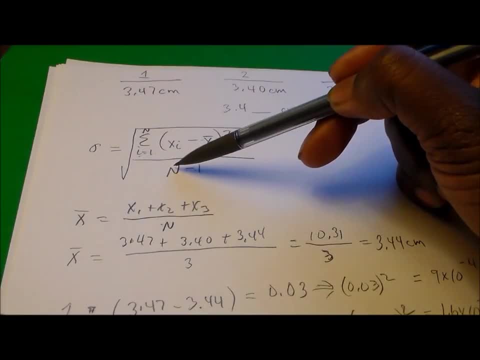 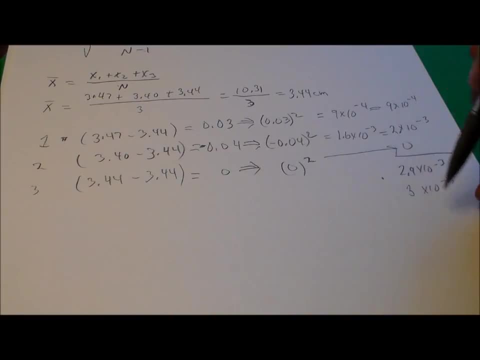 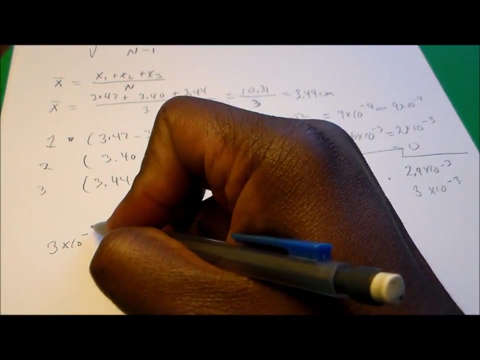 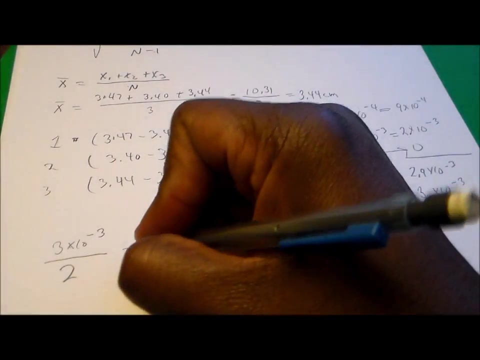 the numerator. now we need to divide that by the difference of the sample minus one. the sample number was three, so three now minus one gives us two. so this is going to be equal to then three times ten, to the minus three divided by two. right, and that gives us then: 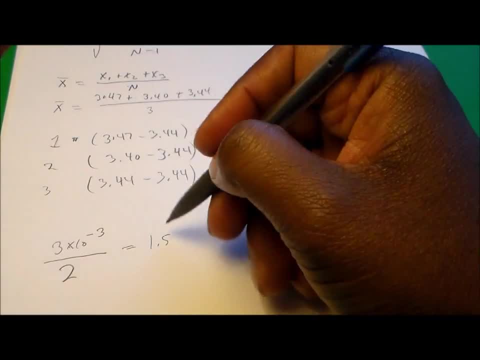 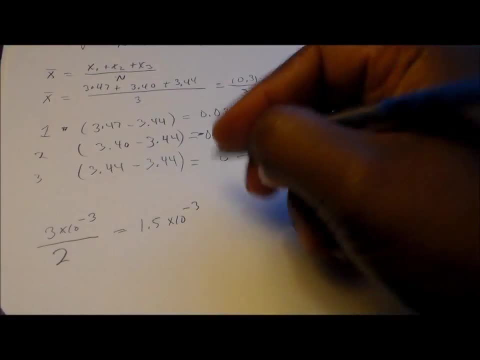 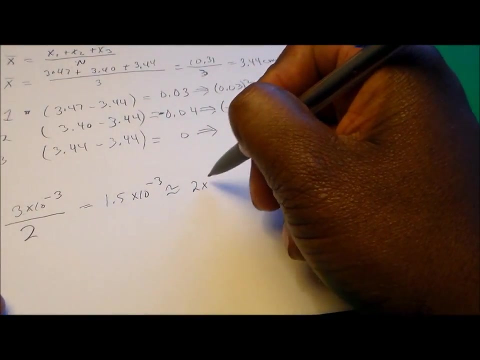 one point five Times ten to the minus three. okay, one point five times ten to the minus three, but again paying attention to significant figures, because we had one significant figure over here. we're going to make that approximately two times ten to the minus three. okay. 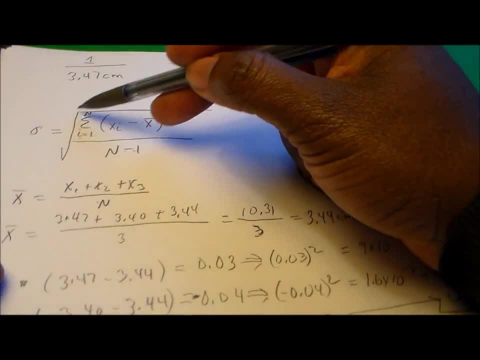 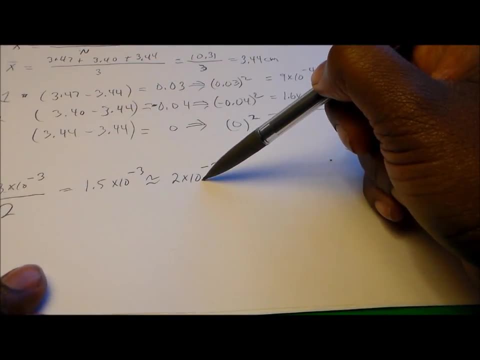 So now we've done everything under the radical sign here we need to go ahead and take the square root of everything, the results of all of that that was below the radical sign. And then that result that was below the radical sign was a two point two times ten to the. 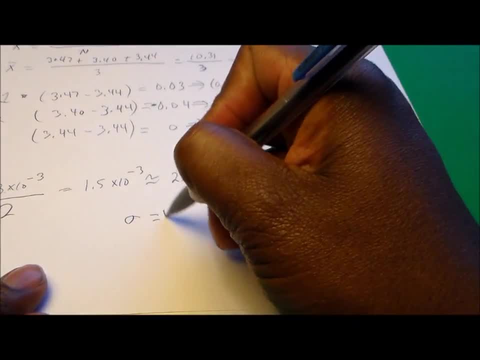 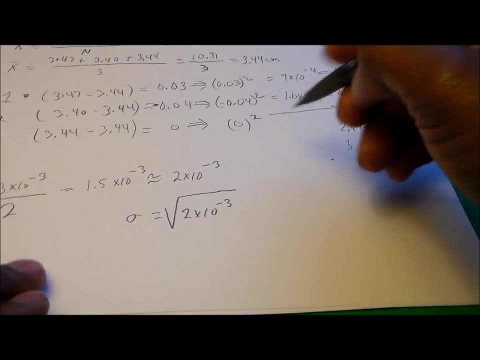 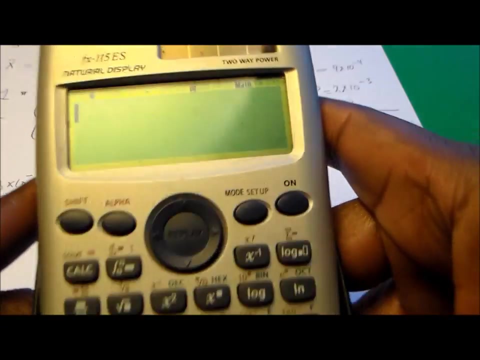 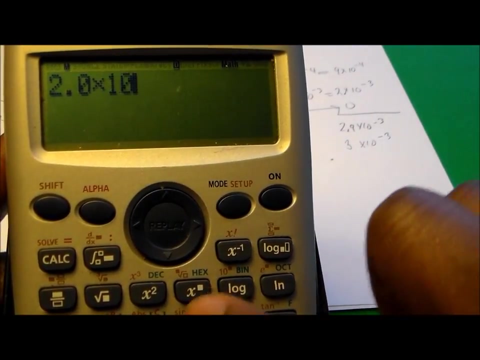 minus three. so therefore, then, sigma is equal to the square root of two times ten to the minus three. Okay, let's see what we end up with when we get that. So I clear my calculator out here. so it's two point zero times ten, raised to the minus. 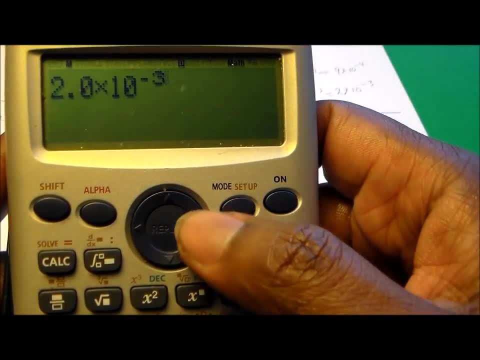 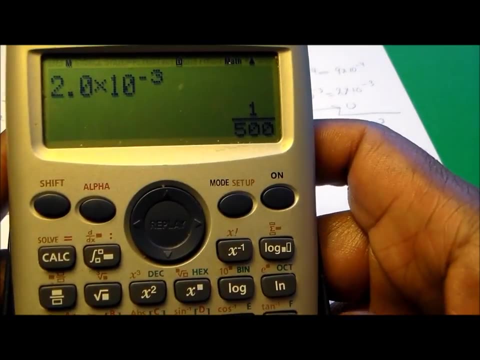 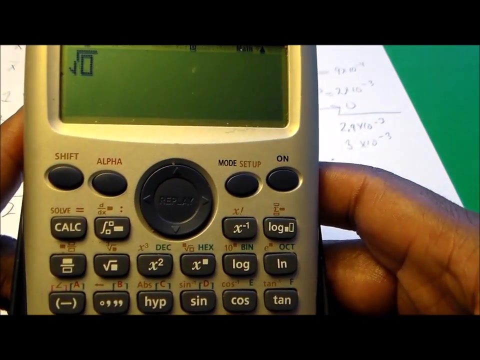 three and let's go back and put the. actually we can go ahead and do this. if we hit equals, it gives us the same thing pretty much, and then we can say that we want the square root. so I hit the square root button up here and then I tell it: I want the square root of my 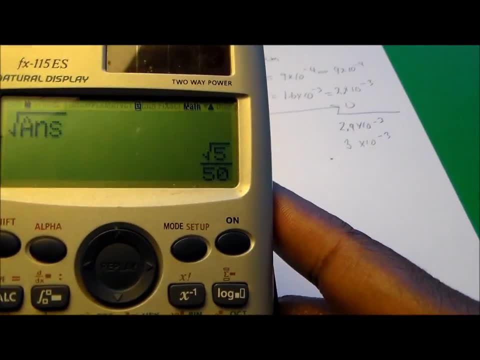 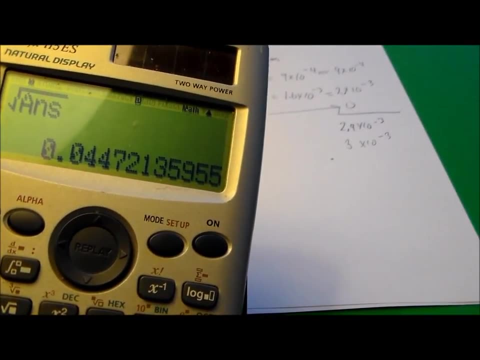 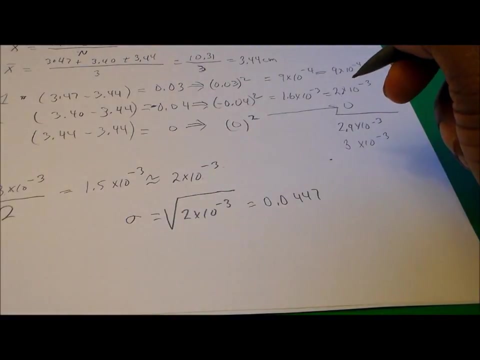 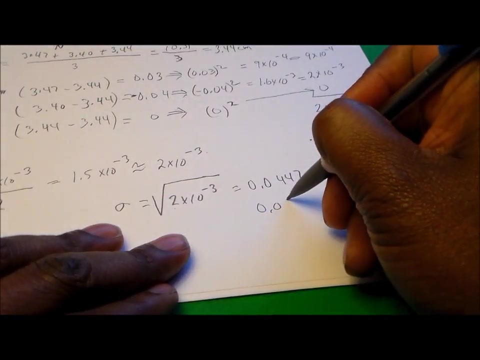 answer. So it's given me a square root of that two times ten to the minus three, and then I need to convert that and it gives me zero point. Zero four four seven. zero point: zero four four seven. okay, but hold on, wait a minute. we only need one significant figure. so this becomes zero point. zero four. okay, zero point. 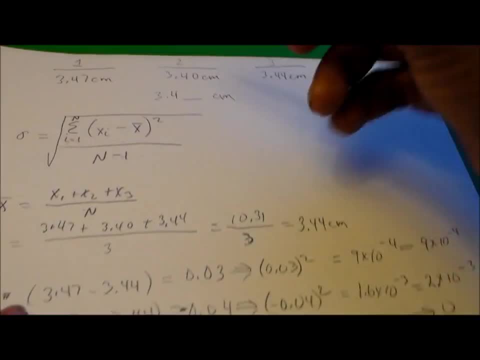 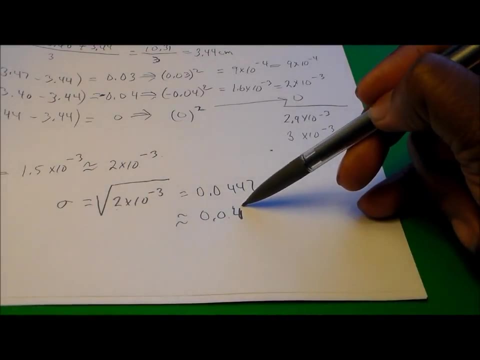 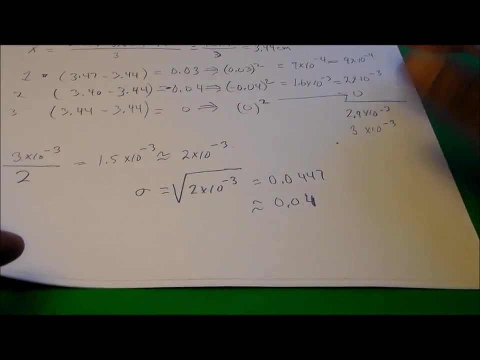 zero four. and also remember, since we were looking for the uncertainty related to this position, then this also makes sense down here, Right, The zero point zero four. okay, So again, we want to express this scientifically. all right, So here's what this here means. 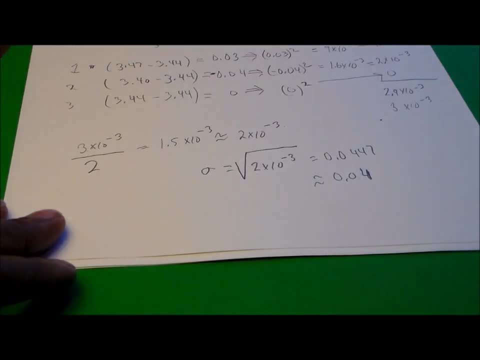 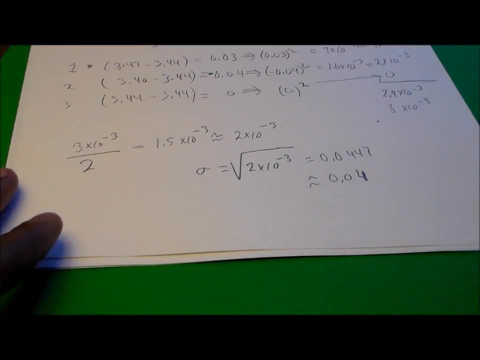 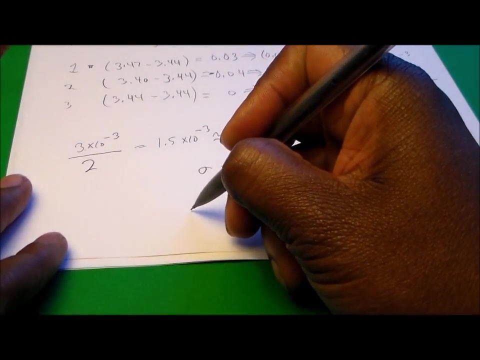 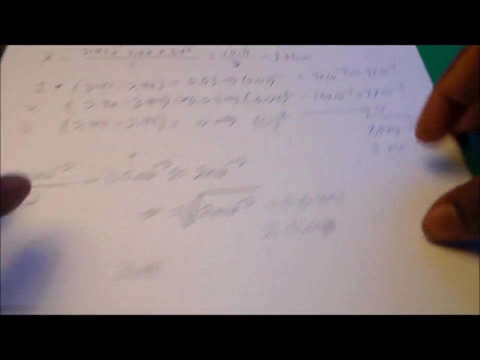 It means that on average, based off of everything, if every measurement that was to continue moving on just in the same estimated, given the same estimated results, Then my average, the average person that takes that does this experiment, will end up having three point four, four, three point four four as the answer, in the way where we got that. 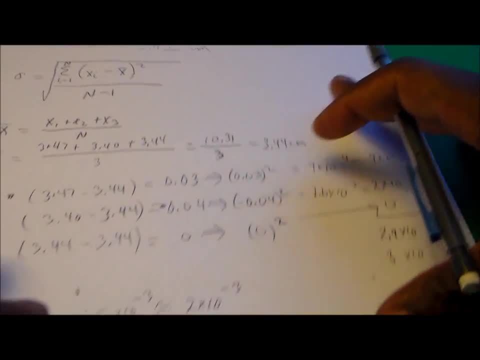 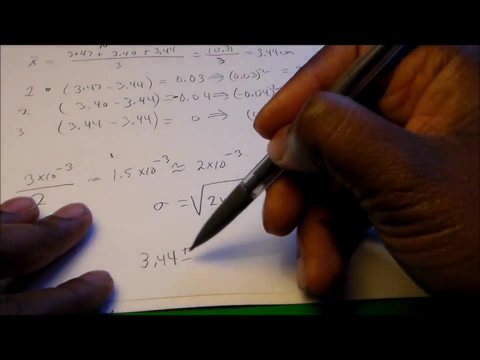 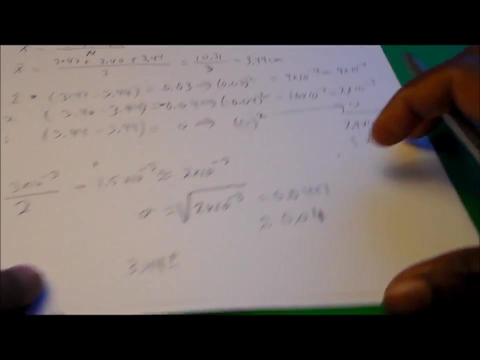 was where we had the egg, from the X bar up here. three point four, four, okay, And then, in terms of their uncertainty, okay, it's going to be then plus or minus, plus or minus the value that we just found here, which was a zero point zero four.